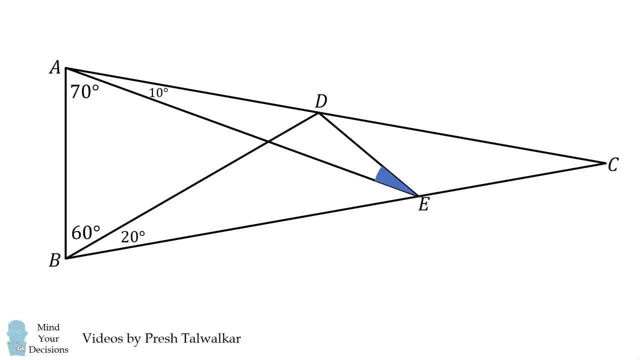 Finally, construct DE. The question is to solve for angle AED marked as X. You're supposed to solve this using only elementary methods. That means no trigonometry. I admit I could not solve this problem and I had to read the solution online, which I will present in the rest of the video. 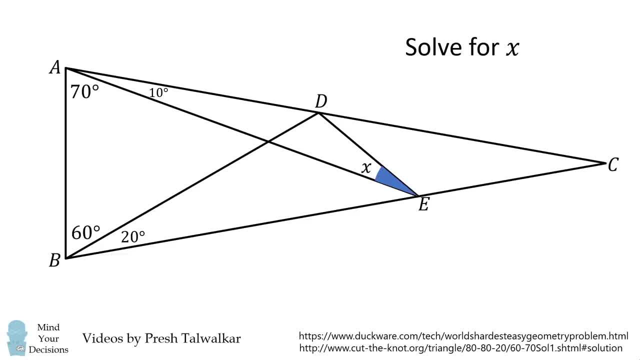 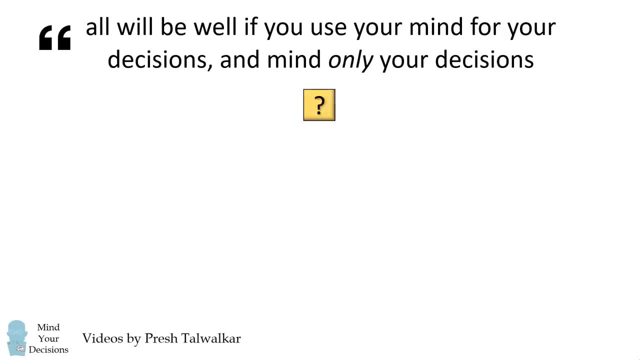 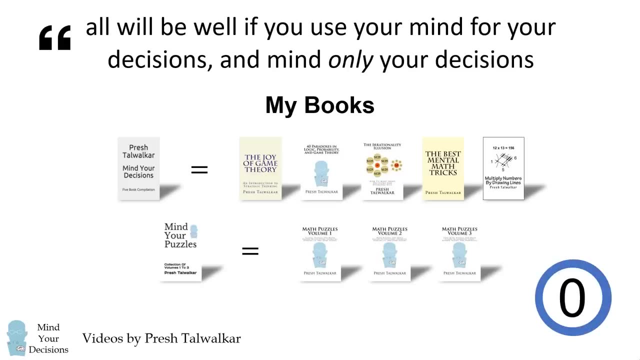 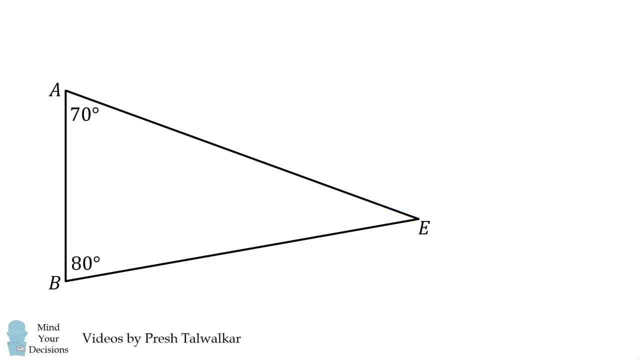 Pause if you'd like to give this problem a try and, when you're ready, keep watching to learn how to solve this problem. We'll get started by focusing on triangle ABE. Angle B is equal to 80 degrees, which means the remaining angle in this triangle is equal to 30 degrees. 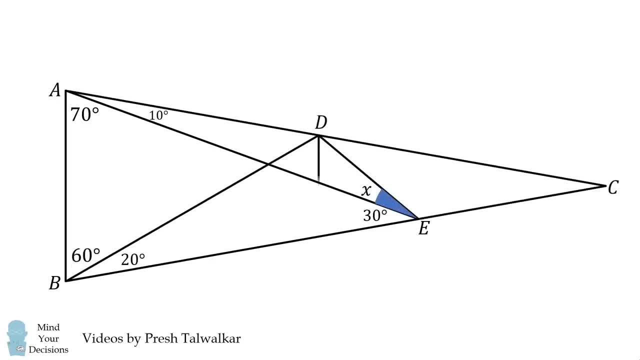 We'll then go back to the original diagram, Construct DF so that DF is parallel to AB. We'll proceed in the following steps. We'll first show that angle DFE is equal to 80 degrees. That'll be the easy part. We then need to show that FD is equal to FE. 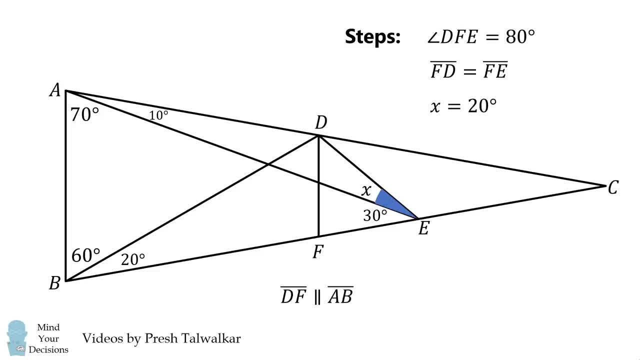 That's the hard part. From there we'll be able to solve that X is equal to 20 degrees. So let's get started. We'll first consider just the following similar triangles. The reason they're similar is because DF was constructed to be parallel to AB. 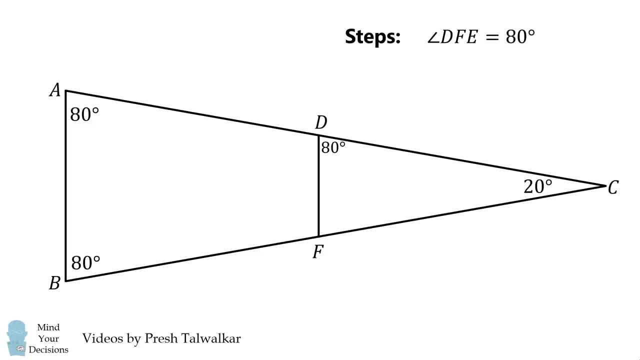 So angle C is equal to 20 degrees, which means the remaining angles will be equal to 80 degrees. We've completed the first part of the proof. We'll now go to the hard part of the proof. We'll first consider the supplementary angles, which will be equal to 100 degrees each. 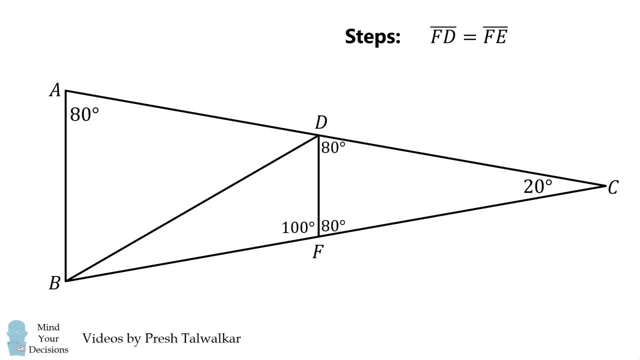 Now again, let's construct BD which divides this angle into 60 degrees and 20 degrees. In this triangle, the remaining angle must be equal to 60 degrees. From here, let's construct AF, which intersects at point G. Notice that this triangle will exactly be congruent to this triangle. 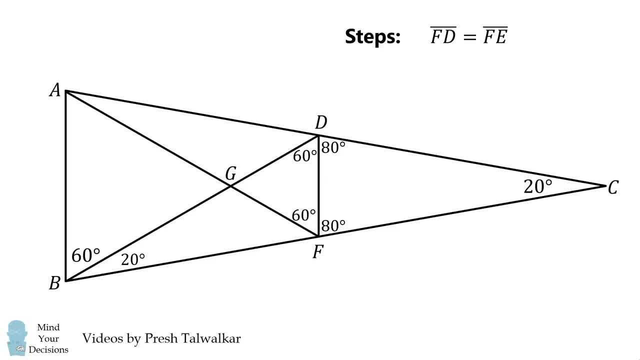 Therefore, angle AFD will be equal to 60 degrees. The remaining angle in triangle FGD must also be equal to 60 degrees, And then by vertical angles we have a 60 degree angle here. Then in triangle ABG the remaining angle must be equal to 60 degrees as well. 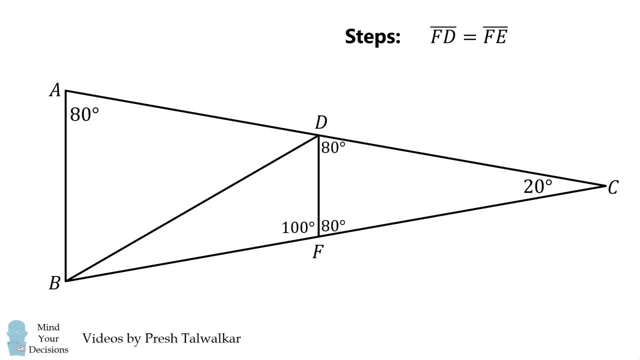 Now again, let's construct BD which divides this angle into 60 degrees and 20 degrees. In this triangle, the remaining angle must be equal to 60 degrees. From here, let's construct AF, which intersects at point G. Notice that this triangle will exactly be congruent to this triangle. 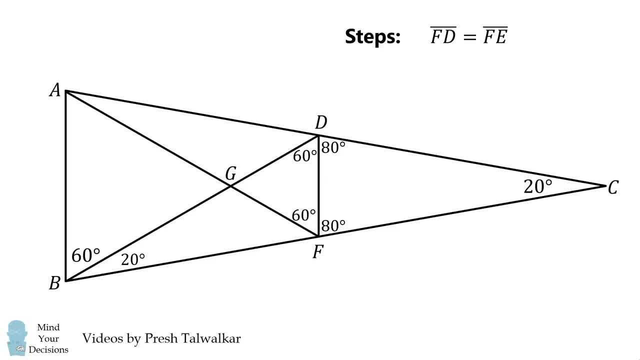 Therefore, angle AFD will be equal to 60 degrees. The remaining angle in triangle FGD must also be equal to 60 degrees, And then by vertical angles we have a 60 degree angle here. Then in triangle ABG the remaining angle must be equal to 60 degrees as well. 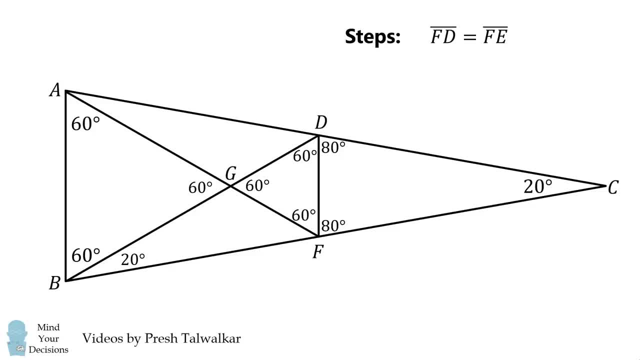 We constructed a couple of equilateral triangles. Furthermore, angle FAD must be equal to 20 degrees, because angle A as a whole is equal to 80 degrees. We've thus constructed an isosceles triangle as follows: The sides opposite the 20 degree angles must be equal to each other. 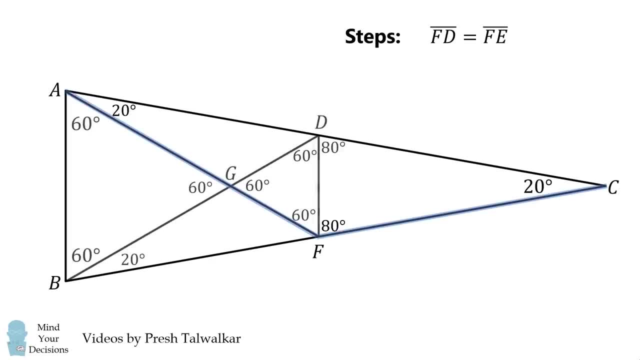 So AF must be equal to FC. Now return to the diagram, and then let's draw in AE again, Recalling that we had a 10 degree angle here from the original information. the remaining angle must be equal to 10 degrees, so that we have a total sum of 20 degrees. 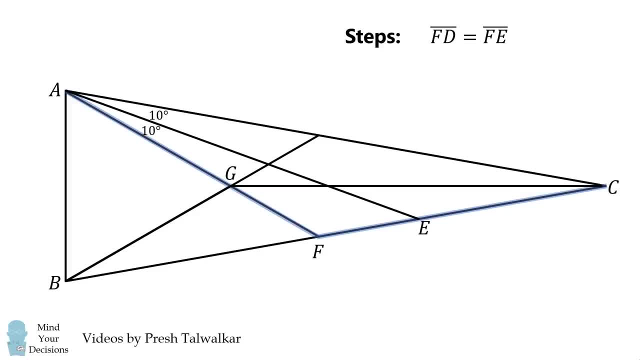 We're then going to bisect angle C, which will intersect at point G. These will be two 10 degree angles. We now have a couple of congruent triangles. Notice that triangle AGC is exactly congruent to triangle CEA. Therefore, AG is exactly equal to CE. 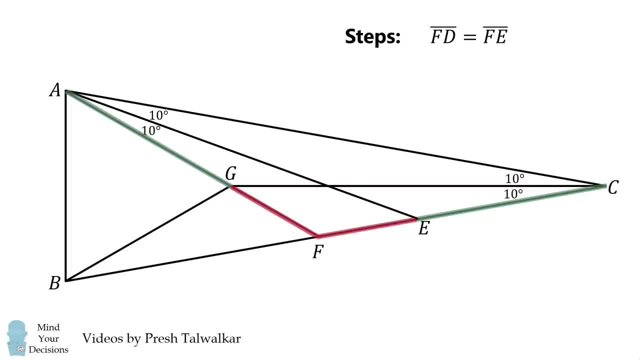 What this means is the remaining segments, FG and FE, will have the same length. From here we go back to the equilateral triangle of FGD and since it's equilateral, we must have FG equal to FD. Consequently, FD is equal to FE and we've proven this part. 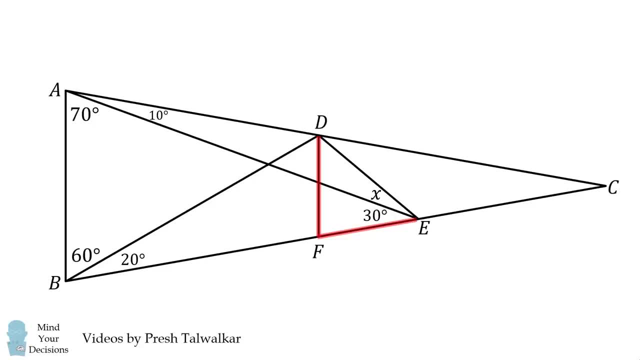 Now, how do we solve the problem? We go back to the original diagram and recall that we calculated that angle DFE is equal to 80 degrees, So we'll now focus on triangle DFE. We have an isosceles triangle where one angle, the vertex angle, is equal to 80 degrees. 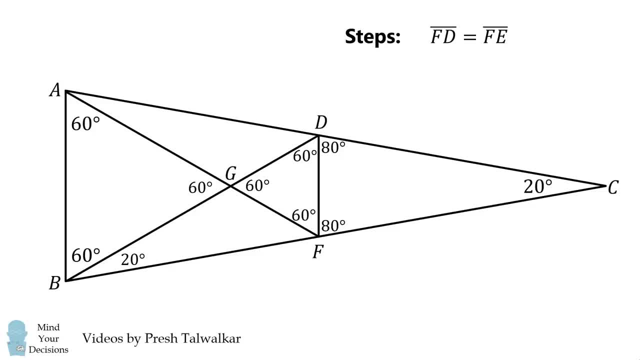 We constructed a couple of equilateral triangles. Furthermore, angle FAD must be equal to 20 degrees, because angle A as a whole is equal to 80 degrees. We've thus constructed an isosceles triangle as follows: The sides opposite the 20 degree angles must be equal to each other. 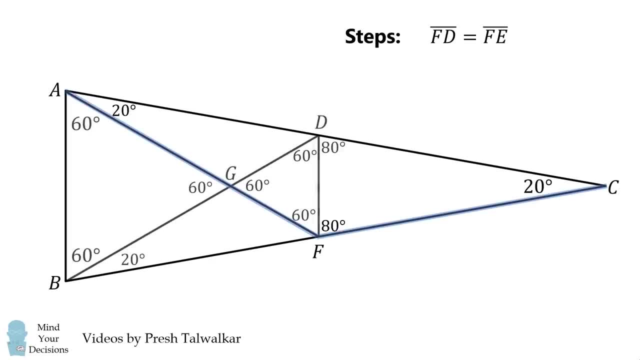 So AF must be equal to FC. Now return to the diagram, and then let's draw in AE again, Recalling that we had a 10 degree angle here from the original information. the remaining angle must be equal to 10 degrees, so that we have a total sum of 20 degrees. 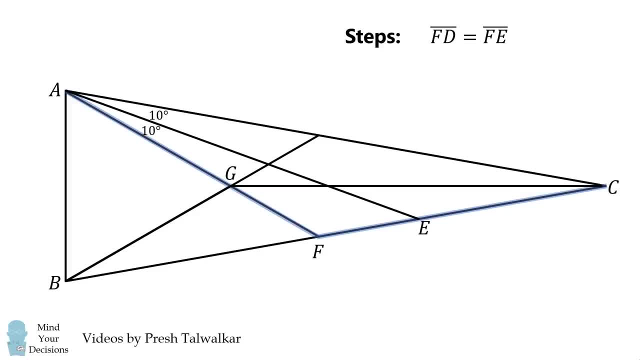 We're then going to bisect angle C, which will intersect at point G. These will be two 10 degree angles. We now have a couple of congruent triangles. Notice that triangle AGC is exactly congruent to triangle CEA. Therefore, AG is exactly equal to CE. 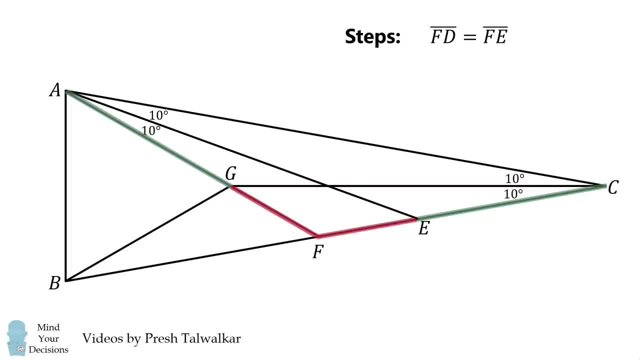 What this means is the remaining segments, FG and FE, will have the same length. From here we go back to the equilateral triangle of FGD and since it's equilateral, we must have FG equal to FD. Consequently, FD is equal to FE and we've proven this part. 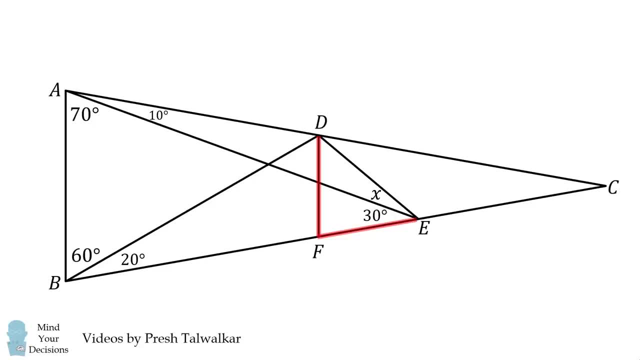 Now, how do we solve the problem? We go back to the original diagram and recall that we calculated that angle DFE is equal to 80 degrees, So we'll now focus on triangle DFE. We have an isosceles triangle where one angle, the vertex angle, is equal to 80 degrees. 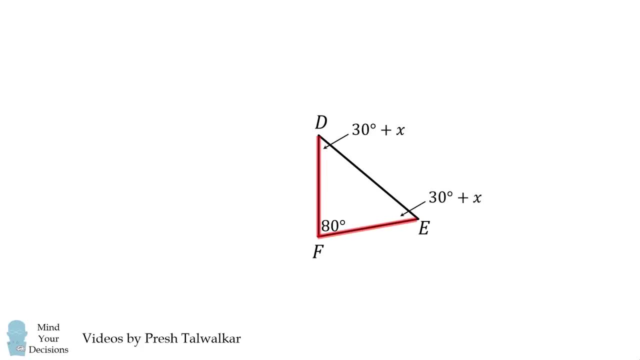 Two equal angles must be equal to 30 degrees plus x. So we have the following equation: 2 multiplied by 30 plus x plus 80 is equal to 180.. We subtract 80 from both sides. We then divide by 2.. 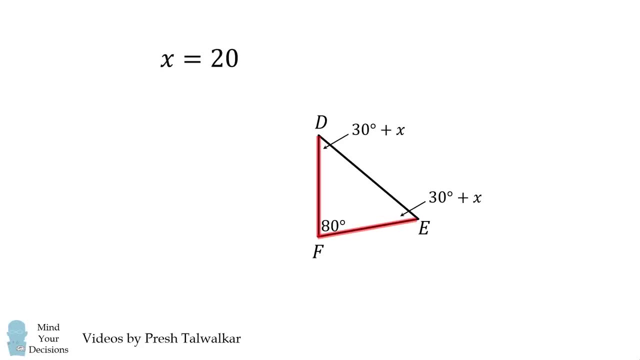 And then we simplify and subtract both sides by 30. And we get that x is equal to 20 degrees And that's the answer. It was a long journey, but it was a satisfying one. Thanks for making Mind Your Decisions. one of the best channels on YouTube. 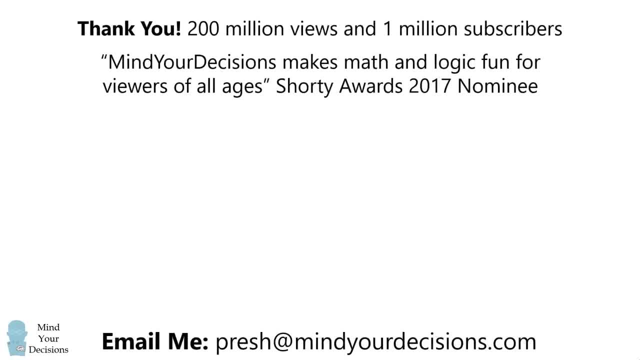 As always, thanks for watching and thanks for your support.